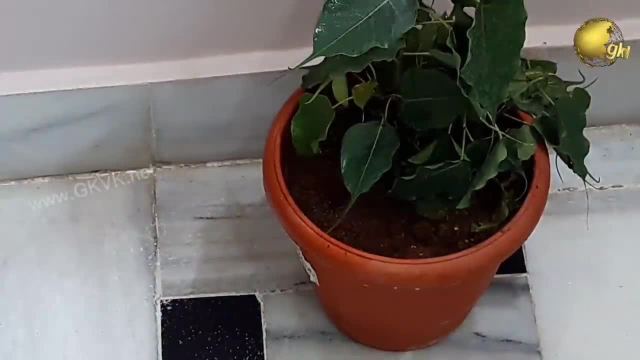 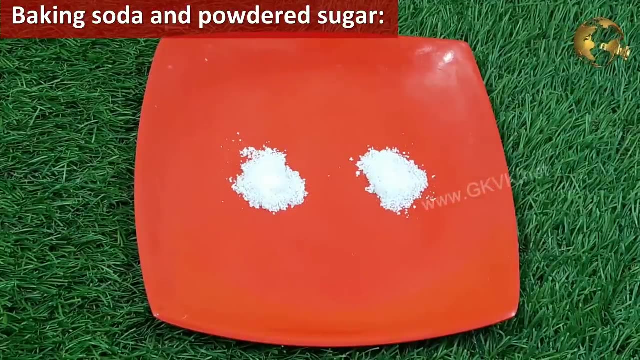 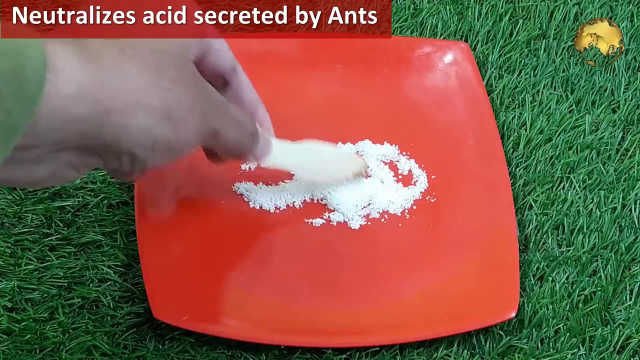 a pinch of salt at the corners of your home or garden. Baking Soda and Powdered Sugar – Ants produce an acid for their defense mechanism To harm them. we can neutralize this acid by mixing equal amounts of baking soda and powdered sugar. You can put this in a container like a lid or plate and keep it in the places where. 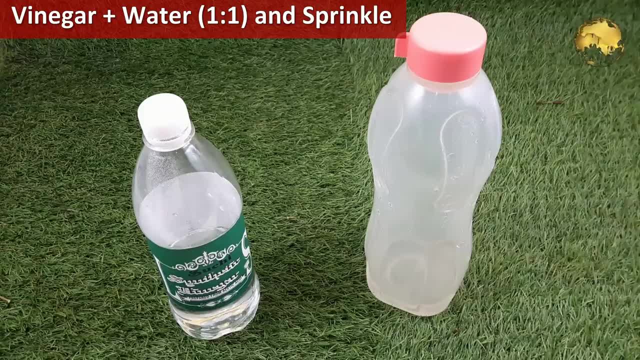 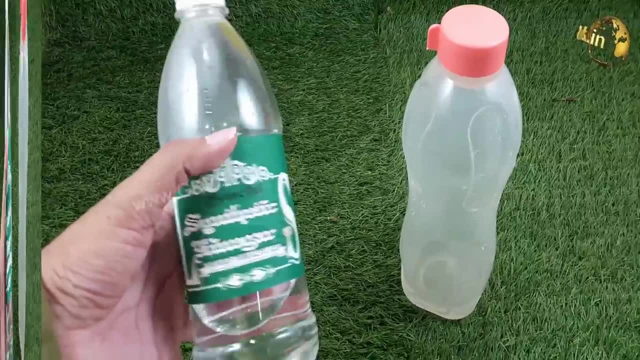 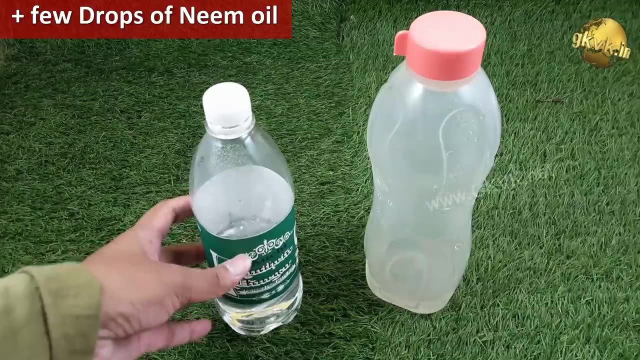 you find ants White Vinegar – It is believed ants cannot bear the smell of white vinegar. Prepare a solution of equal amounts of water and white vinegar. Add a few drops of some essential oil to it. Neem oil drops would really increase its effectiveness. Mix this. 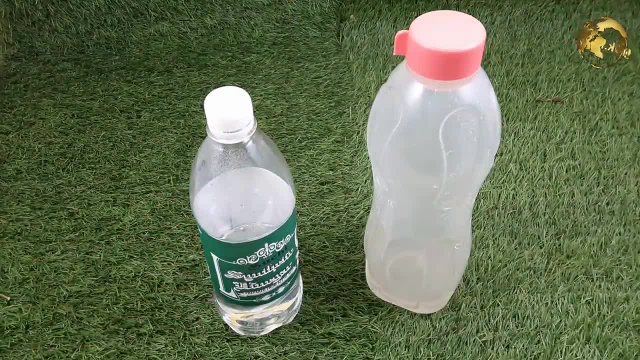 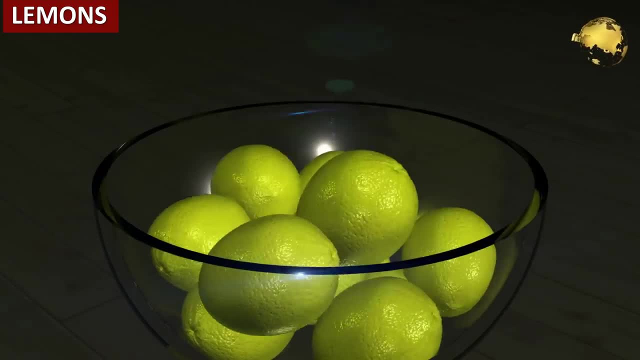 solution. well, Store this solution and sprinkle it. Repeat this if necessary. Lemons – Squeeze a lemon or place lemon peels near ant places. You can also wash your fruits with water that has some lemon juice added to it. Ants do not like the smell of. 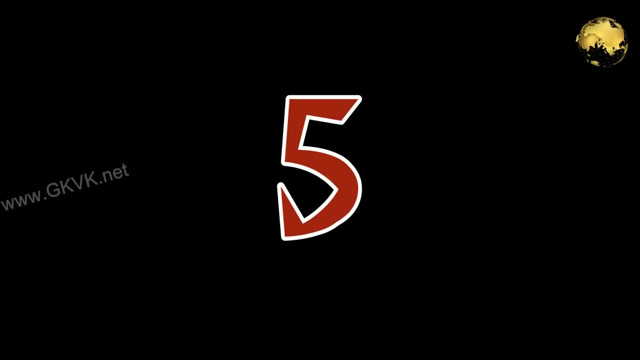 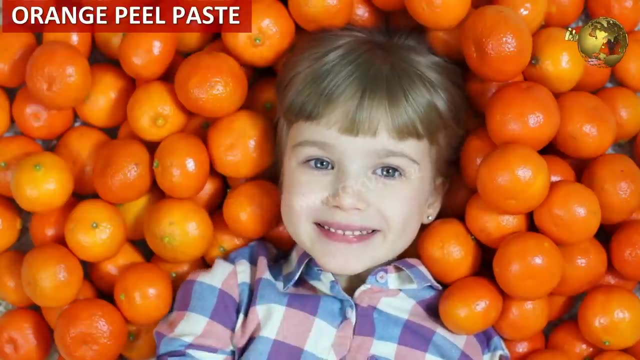 lemon juice. You can also wash your fruits with water that has some lemon juice added to it. Ants do not like the smell of lemon juice. Then, Similarly, Orange Peel Paste – Make a paste of orange peels in warm water and paint this at ant places and the holes of the ants. Then wipe it after 1 or 2 days and then repaint. 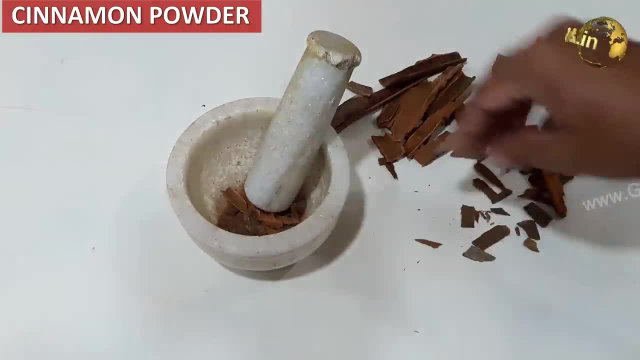 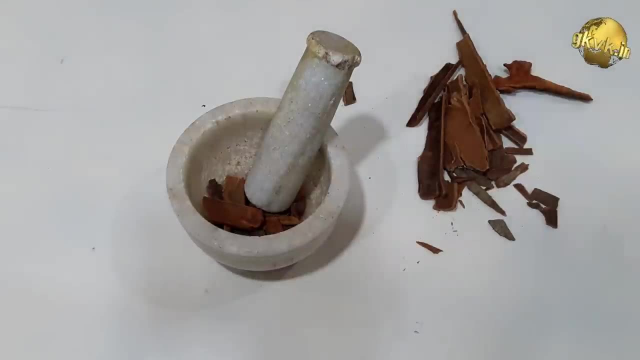 if required, Then Cinnamon Powder – Sprinkling cinnamon powder is a good remedy for ants. You can see the effect immediately after you sprinkle some cinnamon powder. But actually this is not a cost effective method. You can use this only in emergency, when you do not have any. 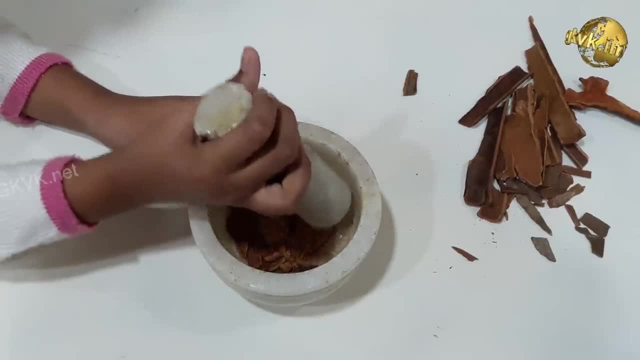 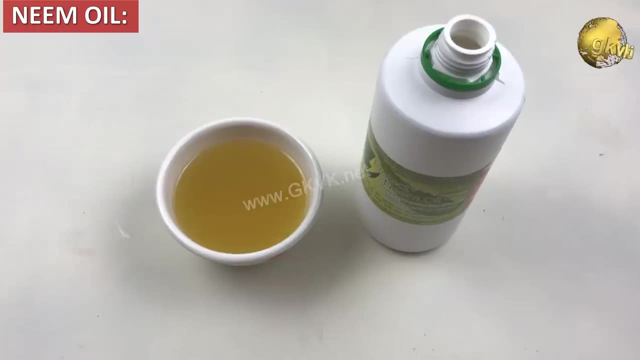 alternate way, Then you can use this only in emergency, when you do not have any alternate way. You can safely sprinkle this in the ant places. You can safely sprinkle this on the soil around your plants. Then Neem Oil – About 10 ml in 1 litre of water. You can sprinkle this on the soil around. 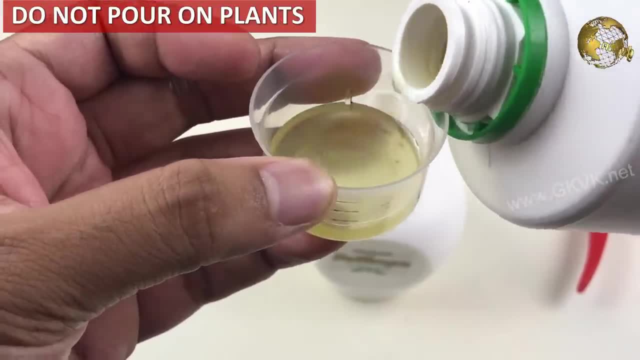 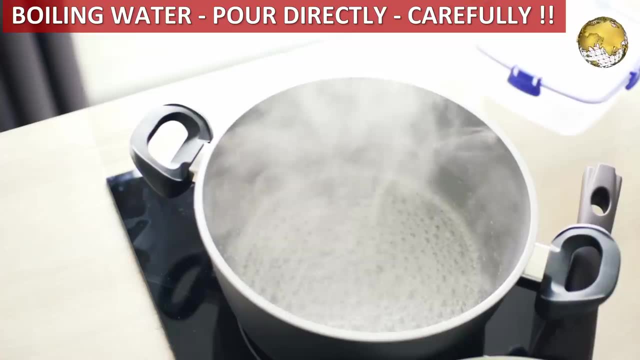 your plants, but not directly on the plants, Because this is double concentration: it can burn the plants. Then Boiling Water – If its feasible, you have to carefully drop boiling water on there residing places. I know it sounds little harsh, but your home and garden are most important to your plants. 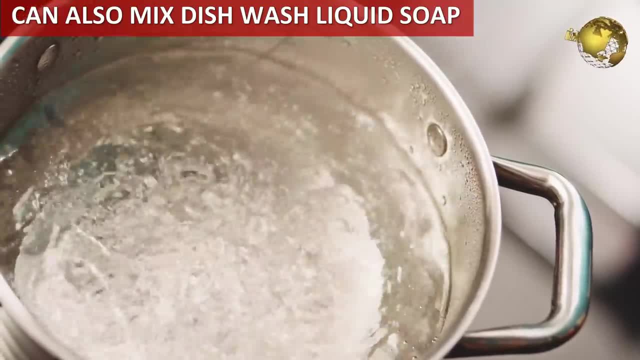 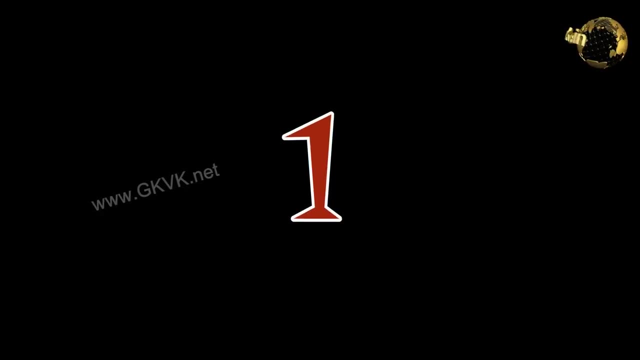 Your home and garden is most important to you and your plants, Then it is a must to keep the plants in your home and garden. If you have more than you than these creatures, You can also mix some dish wash liquid to warm water and spray on them.